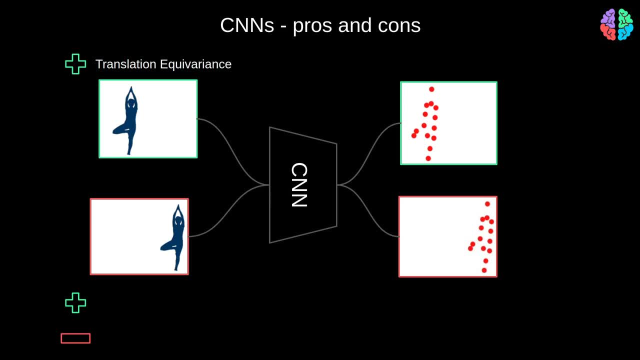 the right in one of the images compared to the other. This very property also helps improve the generalization ability of CNNs, and we can also use augmentation techniques to train using relatively less images. But CNNs don't have that much of a model capacity compared to transformers. 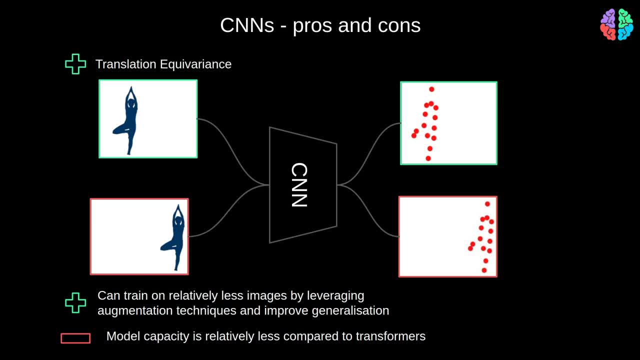 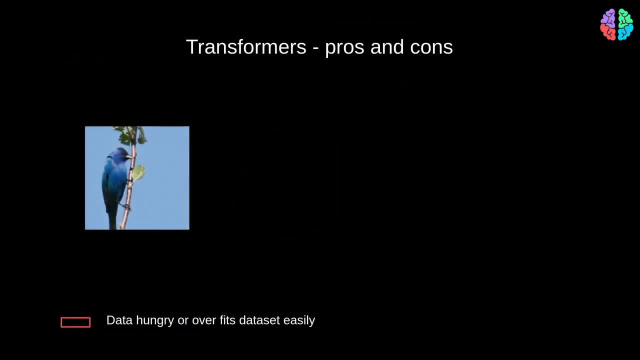 With the kind of data explosion we are going through, we should be able to learn from billions of images, So this is where transformers come in handy. Transformers were originally developed for sequential data, which are like textual inputs, So they have large model capacity. 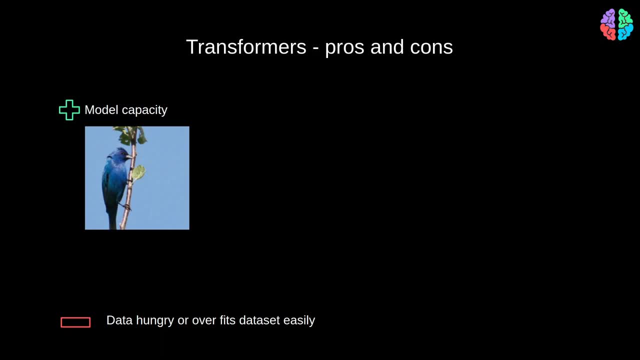 Also, the main building block of transformers is the attention module, and the beauty of attention is that it captures global information in the input. In other words, transformers act as global receptive field. This very good property also acts against us when applied to images. 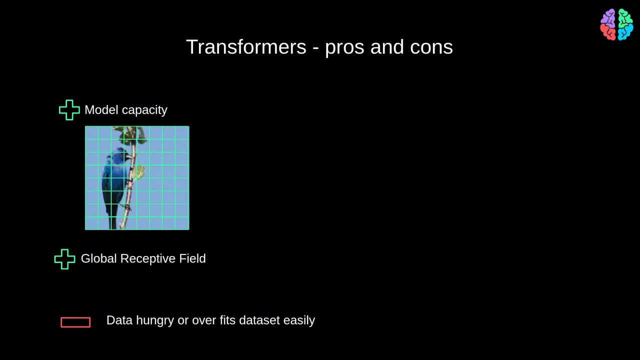 When applied to images, which are two-dimensional data rather than sequential data. Because of the global receptive field, a rotation or a translation augmentation such as this is not too different from the original image, and so transformers tend to overfit the data very easily. This is the main reason we have to train transformers. 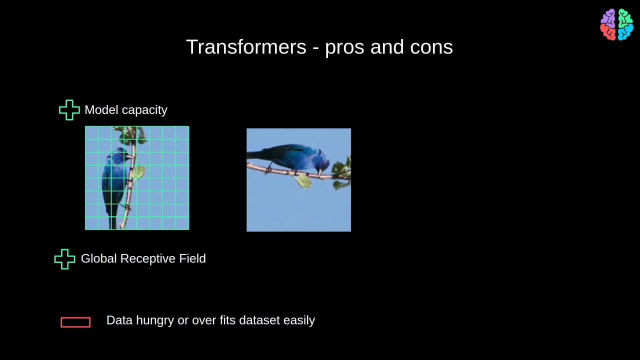 with millions and millions of images, or in other words, transformers are data hungry and can easily overfit the data set. we can make them look like they're plug-inäv. So if, if we can bring together the advantages of CNNs and transformers, 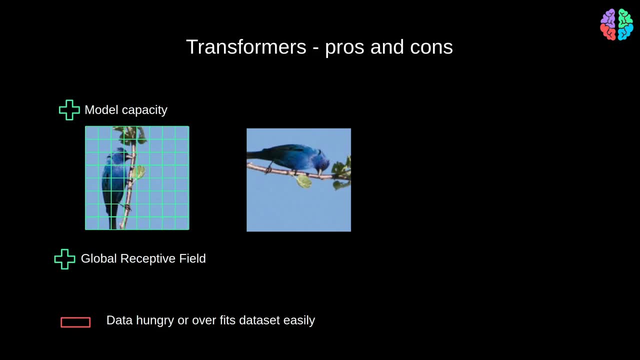 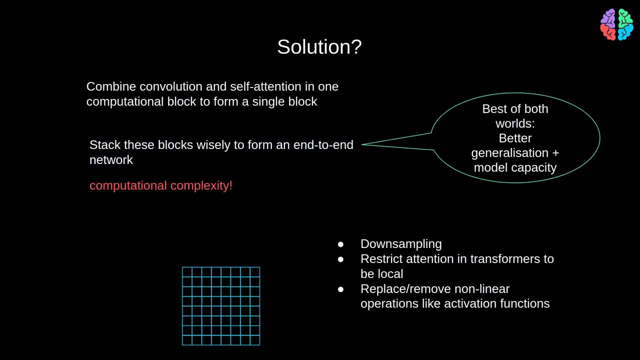 then theoretically we should have a much more efficient network. well, the no sc心 is to combine the conv and transformer blocks into a single block And we can stack the convolution and transformer blocks together. but The biggest bottleneck to this approach is the computational complexity. 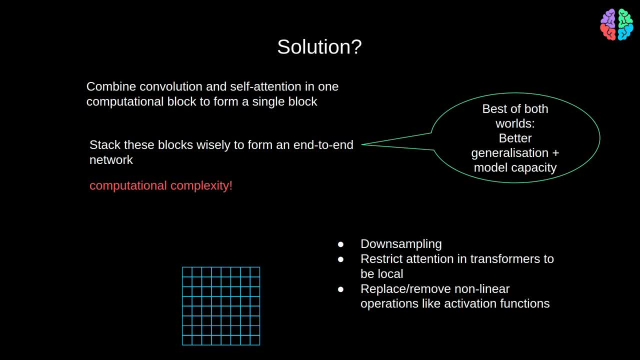 So, as a solution, we can either downsample the images to a lower dimension. In this case, if we take an input image of size 224 by 224,, we can reduce it to say 112 by 112 and then work with. 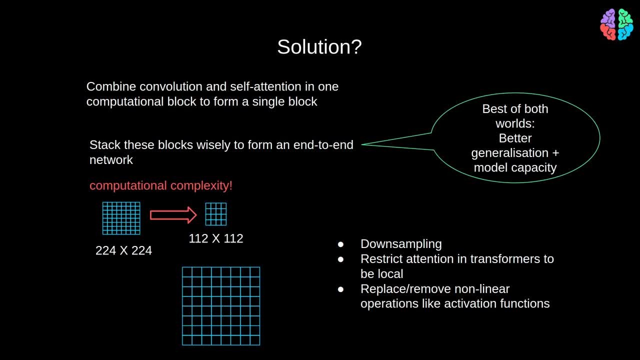 the lower dimension at later stages of the network. Another option could be to restrict attention to local regions instead of being a global region, But then that doesn't make the most out of the transformers. Lastly, reducing or even removing non-linearities like softmax. 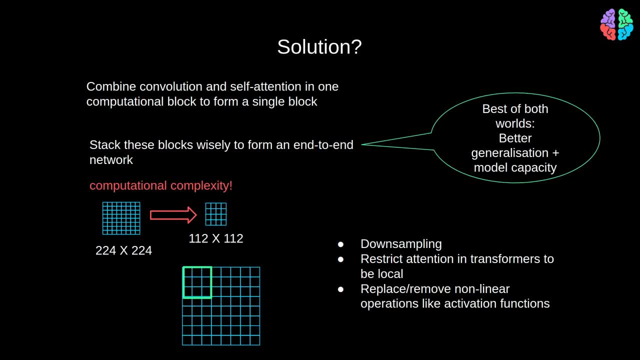 activation can also reduce the computation. The solution chosen in Codenet is that of downsampling, which seems to work far better than the other two approaches. To understand what I mean, let's look at the Codenet architecture and take it from there. Now, this is the proposed architecture of Codenet. 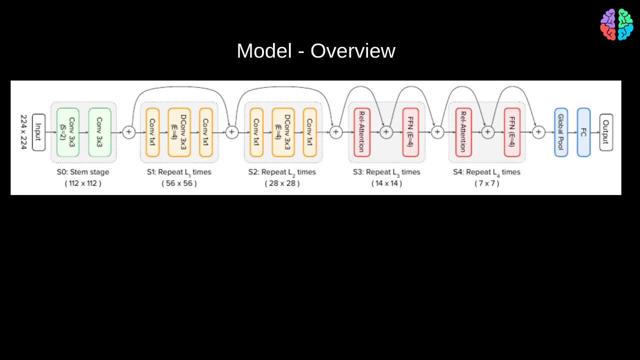 The architecture can be broken down into four parts that are highlighted in different colors. The first is the stem stage, where we have a small network used to scale down the input to a manageable size. The second is the stem stage, where we have a small network used to scale down the. 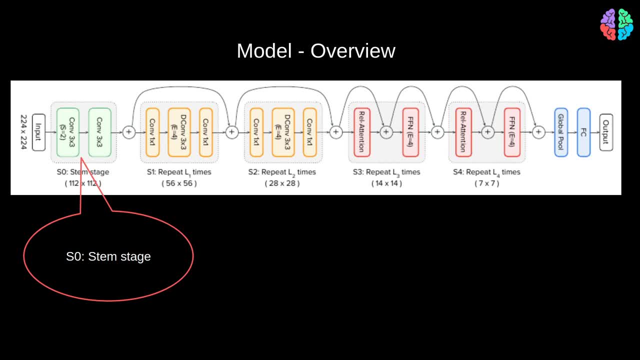 input to a manageable size. The third is the stem stage, where we have a small network used to scale down the input to a manageable size. It can be either a single layer network with a large stripe, as in vision transformers, or it can be a multi-layer network that can be used for the same. 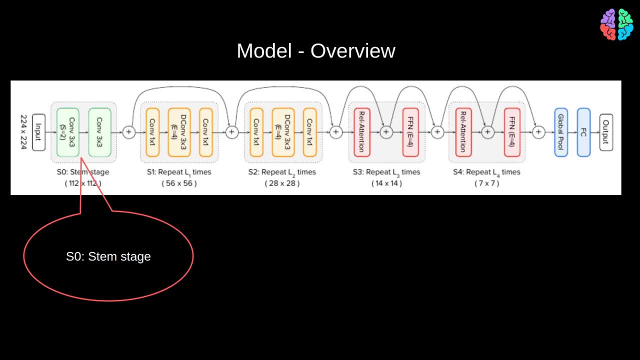 purpose. The next four stages are interesting. There can be convolution blocks or transformer blocks, of course, with attention. In this particular figure, S1 and S2 are convolution blocks, which are shown in yellow, and S3 and S4 are transformer blocks, shown in red. Now you may ask: 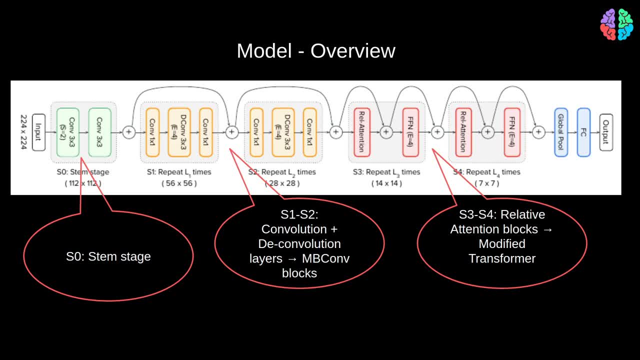 what's, inside these stages, that makes this network special, And before we look into the details, let's just keep in mind that what we see here is two conf and two transformer blocks, But it's also possible to change these numbers and experiment with different combinations. 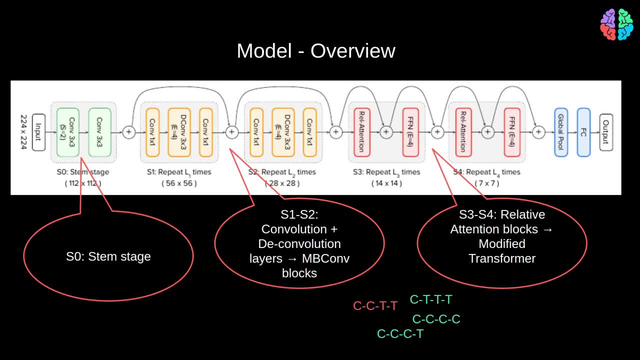 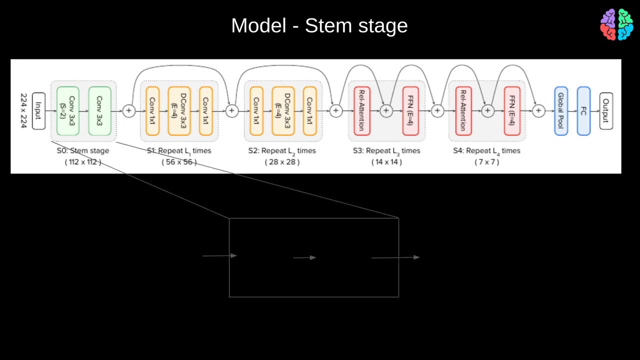 like one convolution block and three transformer blocks, or three convolution block and one transformer block, etc. So now let's look into each of the stages one by one. The purpose of the stem stage is to simply reduce the input to a manageable dimension so that we can do heavy computations, like attention computation, easily on the lower dimension. 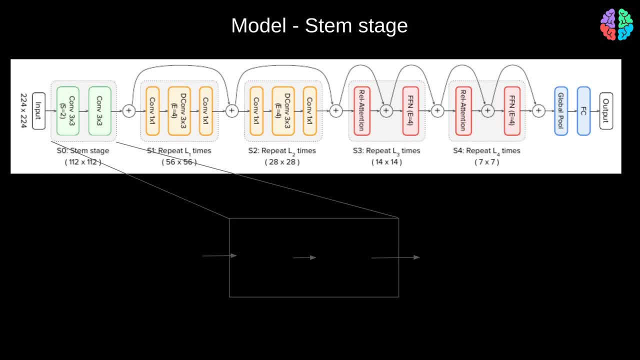 This stem stage has a sequence of conf, patchnorm and activation layer like GELU, as shown here, Even though it's possible to have a single downsampling layer, like in vision transformer. we have illustrated a simple two-stage convolution block with a stride of 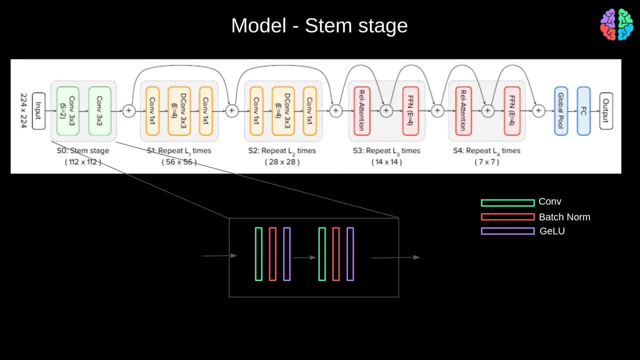 two by two. So if we take an input image of size 224 by 224, the stem stage should be able to halve the input to a size of 112 by 112.. So the stem stage is that simple. Let's move on. 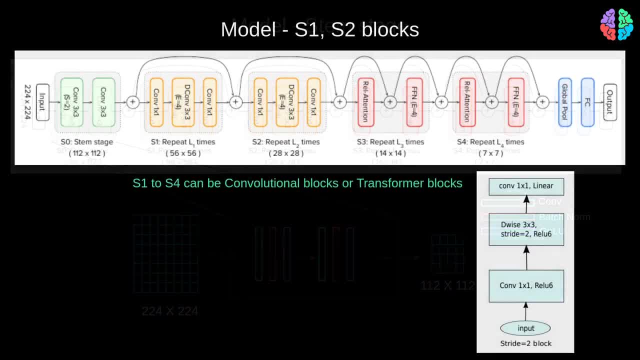 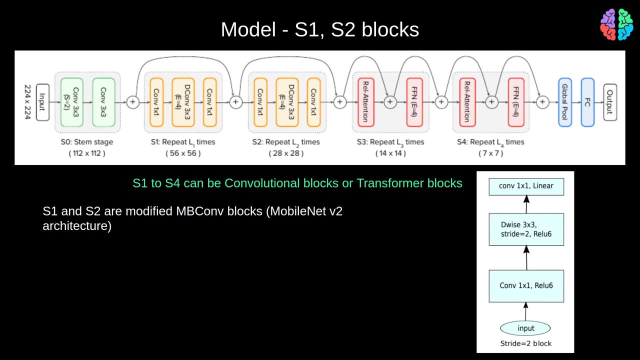 to the convolutional stages S1 and S2.. For the convolutional block, they have chosen MBConv blocks which were introduced in the MobileNet version 2 architecture. So let's see what they have done with the MobileNet version 2.. First, for the nonlinearity: 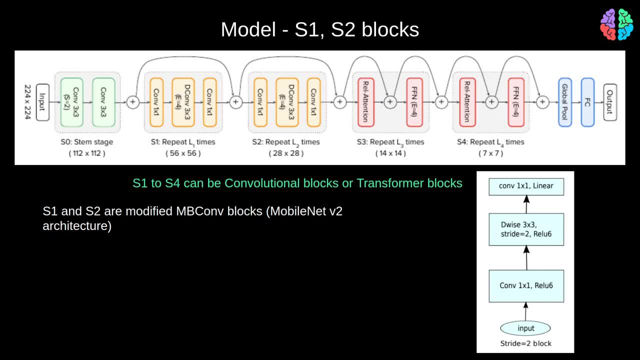 they have introduced the GELU nonlinearity in place of ReLU6 nonlinearity. The next change is that they simply use convolutions instead of depth-wise convolutions for the downsampling stage of the network. This they say that the depth-wise convolution is slower for small networks. 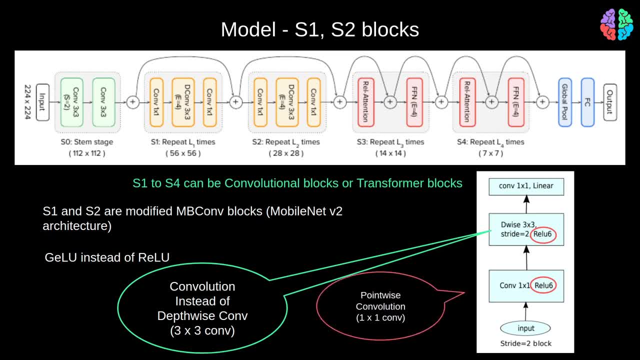 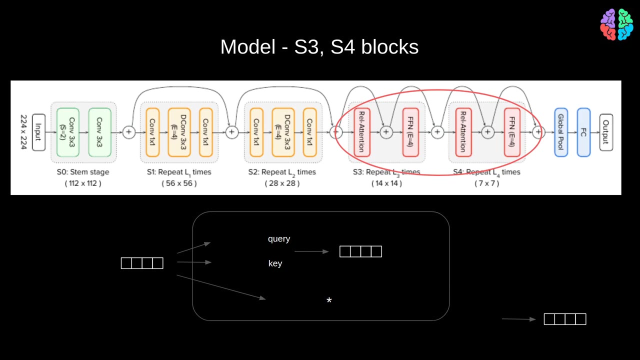 There is no change to the point-wise convolution of the MBConv block and there's also no nonlinearity for the conv layer With those changes to the MobileNet architecture. let's move on to the relative attention which happens within the transformer block, which is stages 3 and S4. Attention is the main component of transformer block. 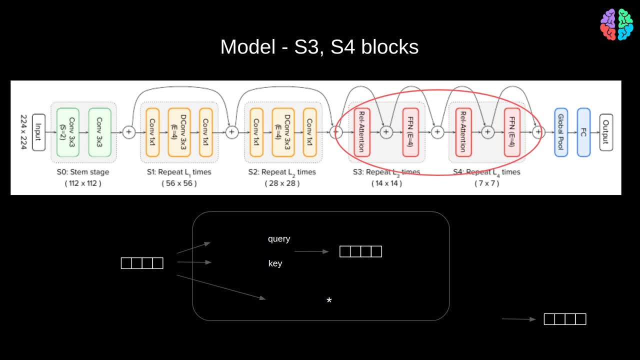 What happens in an attention block is that the input is first split into three components, namely query, key and value. The dot product of query and key is treated separately to that of the value. As we are dealing with relative attention, we introduce a learnable parameter p. 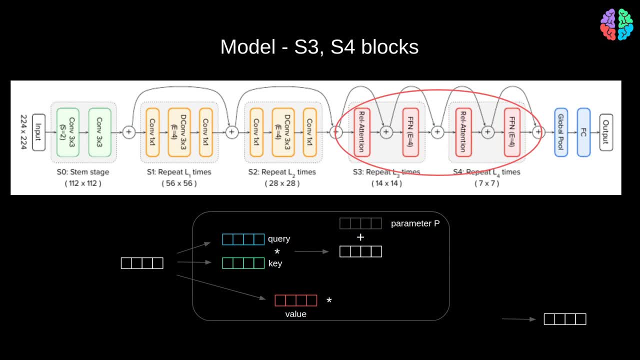 used to compute a relative bias which is added to the dot product of query and key As the next step. the result is put through an activation function like softmax activation. The dot product of query and key is treated separately to the dot product of query and key. 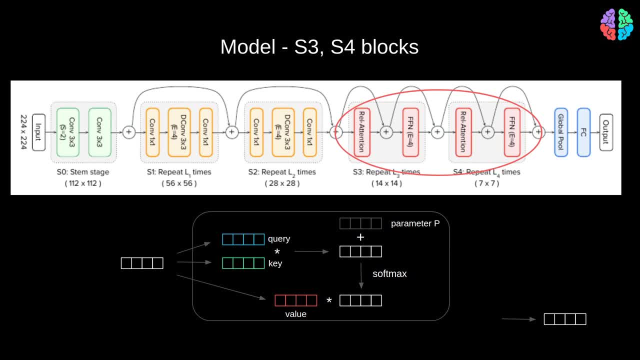 The dot product of query and key is treated separately to the dot product of query and key And finally multiplied with the value to get the output of the attention layer. Now this is the attention module. Separately, the input is passed through a feed-forward network. 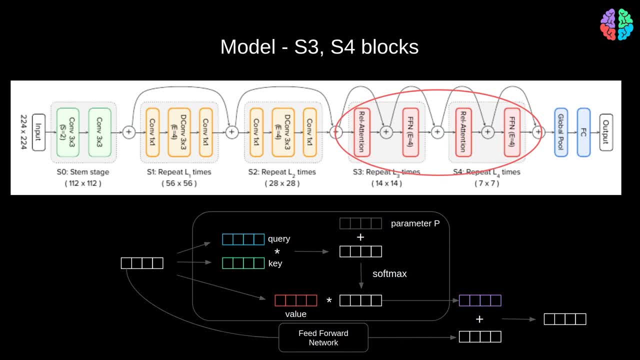 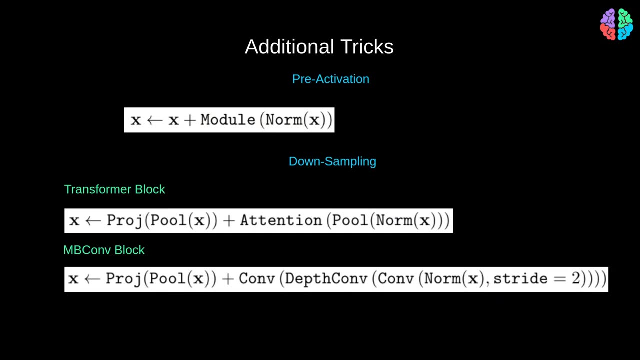 which is a Wendler neural network, and the sum of the two inputs is the output of the transformer block. In addition to these changes, they do have some minor tricks, like the pre-activation which we will see in the next. So pre-activation is the first trick. 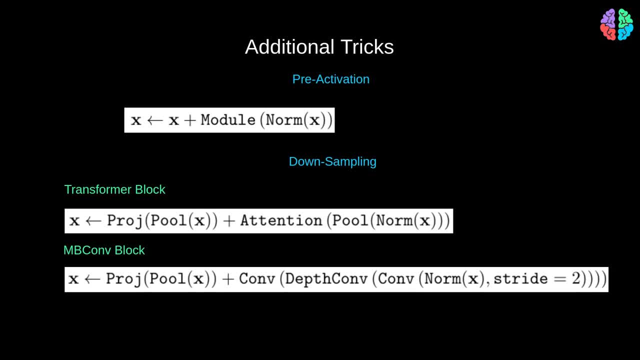 All that it means is that we first normalize the input with batch norm or layer norm and pass it through our module, But finally, and most importantly, we add the output of the module directly to the input. So this is somewhat like a residual network and suddenly your entire block. 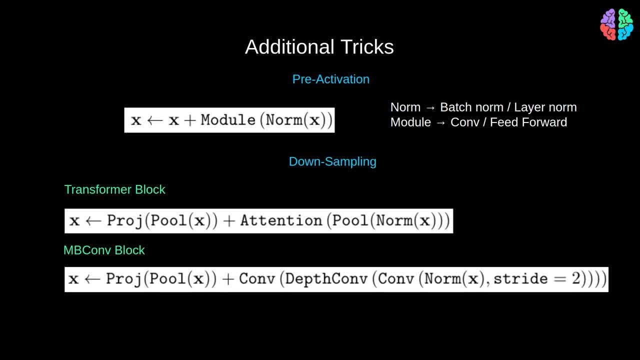 learns more from the residue than from the input. This trick is applied at each and every stage of the network. And then they also have some downsampling, which seems to keep a check on the computation. The choice of downsampling is pooling, both for the transformer and the nbcon block. 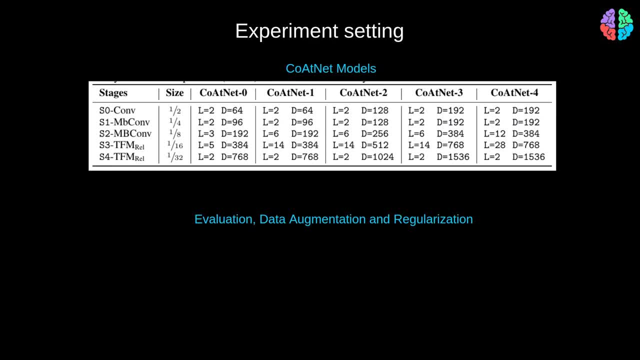 Now on to the experimental setting With the same model, architecture and tricks we just saw. the authors simply increased the number of blocks L and the depth D to create variations to the coordinate architecture and named them coordinate 0 to coordinate 4.. This table just shows different values for L and D for coordinate architectures. 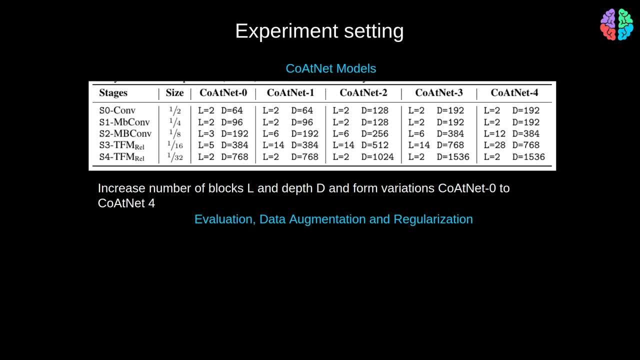 In terms of the evaluation, they mainly used three datasets, namely ImageNet 1k, which is a dataset of size 1.3 million, and then ImageNet 21k, which is a dataset of about 12 million. Finally, they use a proprietary dataset, JFT, which is about 300 million images. 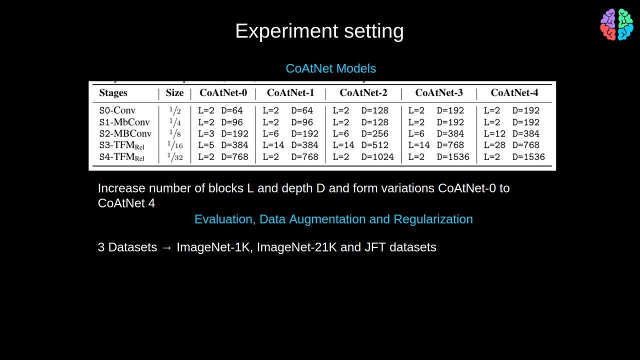 They train on these datasets and finally fine tune on ImageNet 1K. Obviously, to achieve good results, we need to use augmentation and regularization techniques. So for augmentation they use rand augment and mixup, which is becoming very common recently, And for regularization they use stochastic depth label smoothing and weight decay. 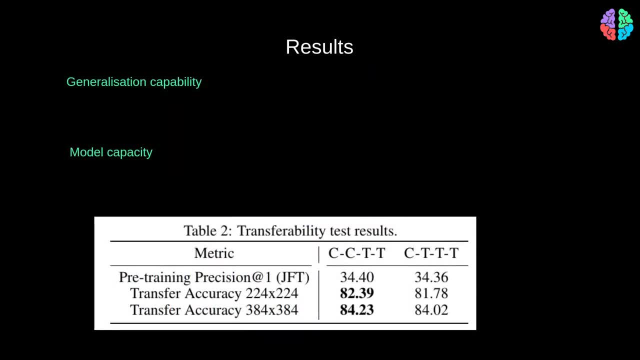 Onto the results. The main reason for developing Codenet architecture is to improve the generalization and model capacity simultaneously for a single network. So it's worth studying systematically the different combinations of conf and transformer blocks In terms of generalization. the more the convolutional layers, the better the generalization should. 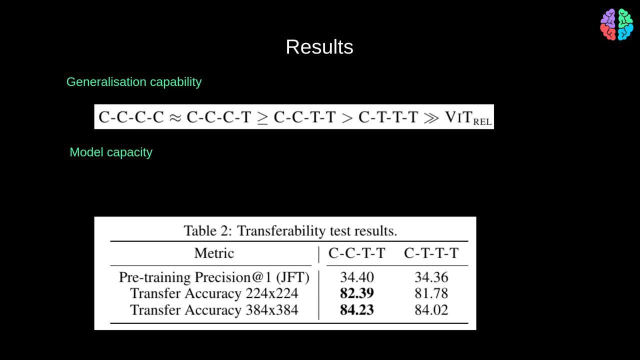 be. The experimental results indeed show exactly the same. As transformers have more model capacity, the more the transformer blocks, the better the capacity should be, And the experimental results indeed agree with this theory. The last thing they study is the transfer learning capability of the network. 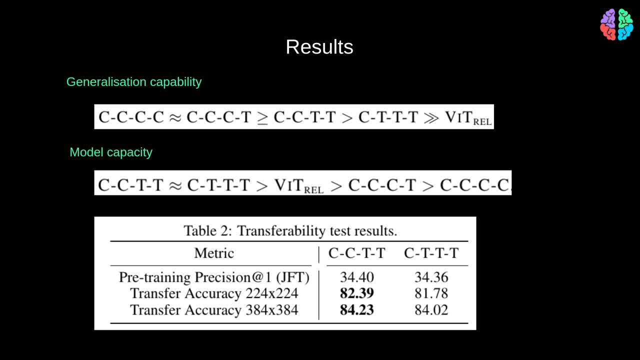 For this they train a network on JFT dataset and transfer to the ImageNet 1K dataset. The model with two conf and two transformer blocks is the winner here, So they have chosen this setup as a standard building block for the Codenet architecture. 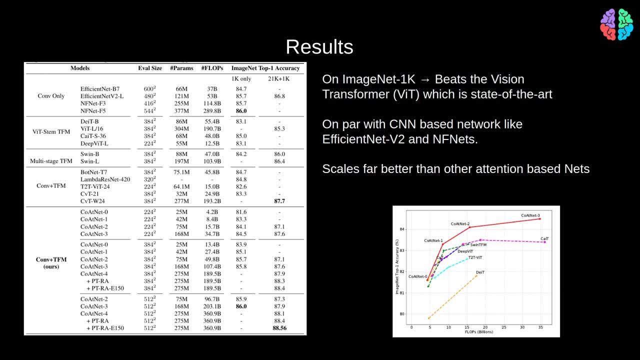 In our experimental setting we mentioned. they use three datasets To report the results. they train on these three datasets and fine-tune on ImageNet 1K. So these are the accuracies on ImageNet 1K. The main thing to note here is that they use three datasets. 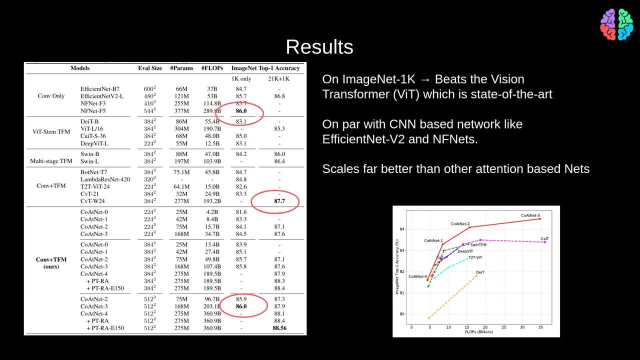 The main thing to note here is that they train on these three datasets and fine-tune on ImageNet 1K. The main thing to note is that the results of Codenet match that of the accuracies we get with convolutional architectures. The results also beat the accuracies we can achieve with image transformers. 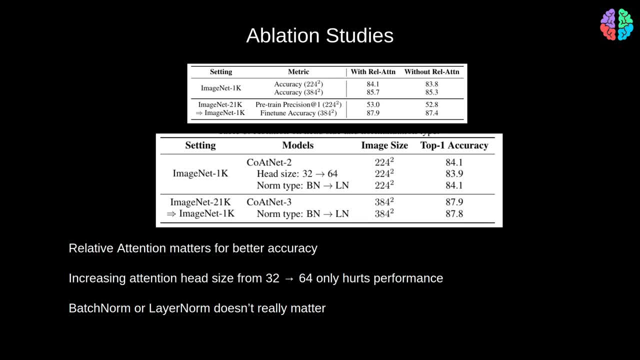 In terms of the ablation, they first study the significance of relative attention in the network. So they experiment with and without the relative attentions, And the results indicate that the relative attention module does bring higher accuracies. They also study the significance of the size of the attention head.